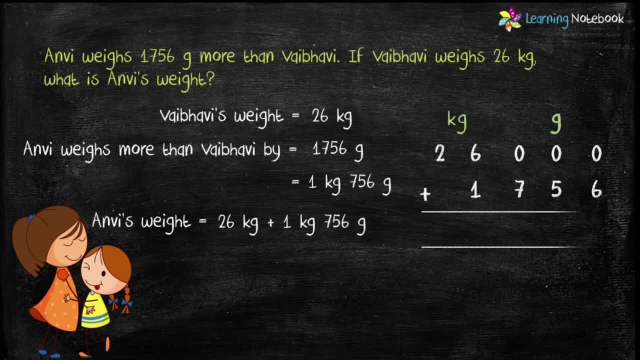 0 plus 6 equals to 6, 0 plus 5 equals to 5, 0 plus 7 equals to 7, 6 plus 1 equals to 7, and 756 g. So let's add them. 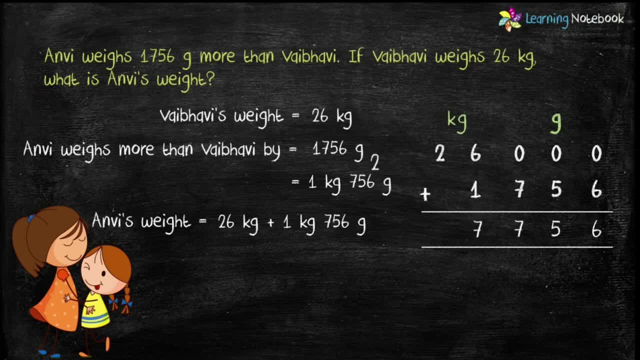 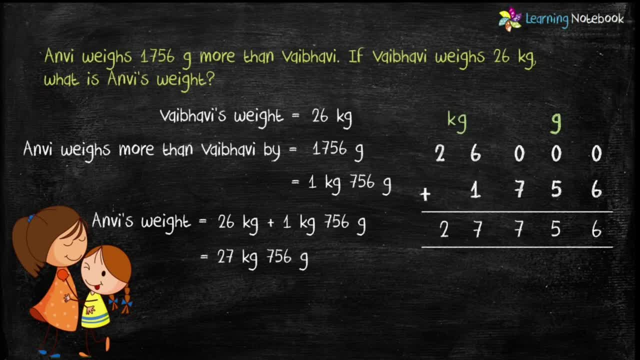 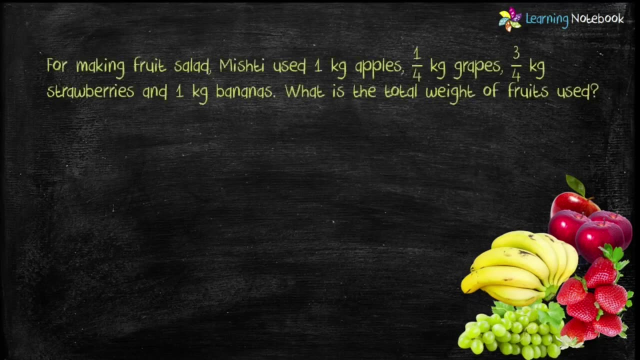 so we get the answer as 27 kg 756 g. Let's write the answer statement: Anvi's weight is 27 kg 756 g. Question 2 is for making�를 fruit saladathy used 1 kg apples, 1 by 4 kg grapes, 3 by 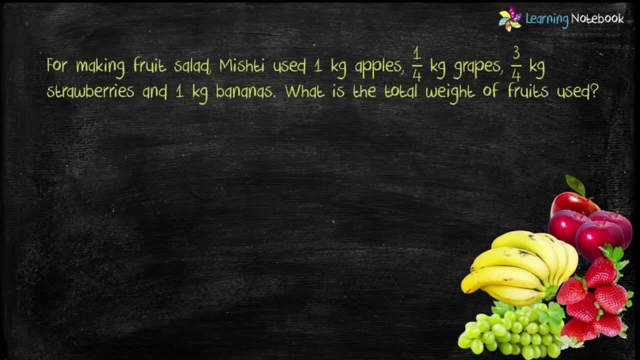 4 kg strawberries, 1 kg apples and 1 kilogram bananas. So what is the total weight of fruits used by Mishti? Let's write the statements. Weight of apples used is 1 kilogram. Next, weight of grapes used is 1. 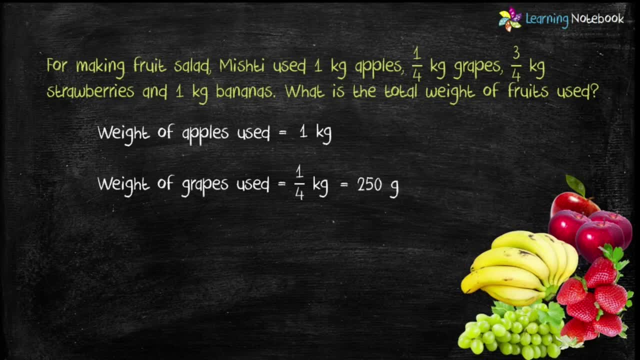 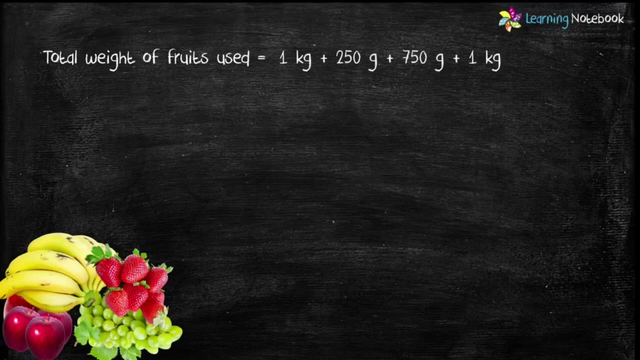 by 4 kilogram, which we know is equals to 250 gram. Then weight of strawberries used is 3, by 4 kilogram, which is equals to 750 gram, And weight of bananas used is 1 kilogram. Now to find the total weight of fruits used, let's add the weight of all these 4 fruits. 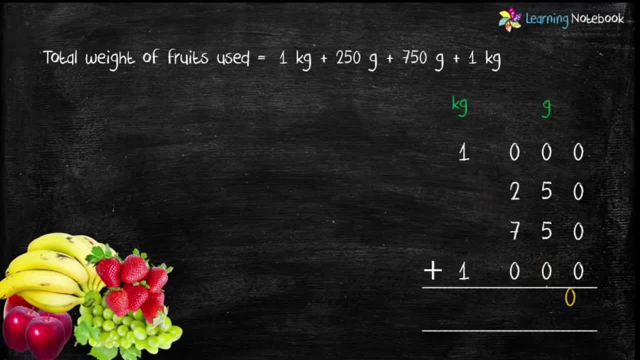 Students while adding, make sure that weights are written properly. That is, weight in kilogram is written correctly. Weight in gram is written under kilogram unit and weight in gram is written under gram unit, So we get the sum as 3 kilogram. Therefore, the answer statement is total weight of fruits. 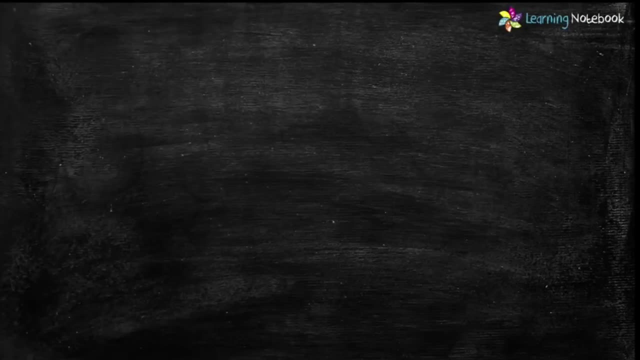 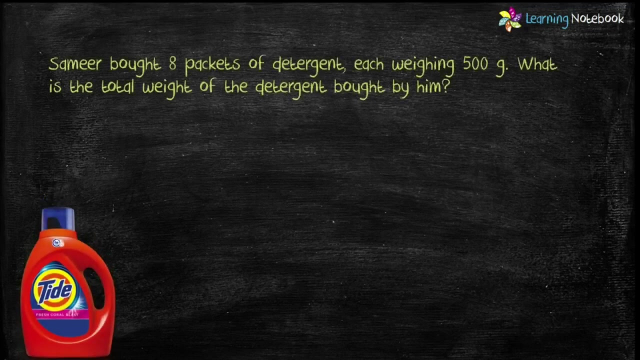 used is 3 kilogram. Next question is: Sameer bought 8 packets of detergent, each weighing 500 gram. What is the total weight of the fruits used Detergent bought by him? Students, let's write the statements: Weight of each packet. 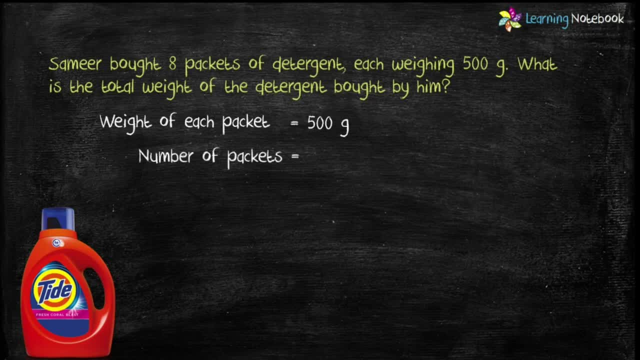 is 500 gram. Number of packets bought is 8.. Therefore, total weight of these 8 packets is 500 multiplied by 8.. So let's multiply it: 8 into 0 equals to 0.. Again, 8 into 0 equals. 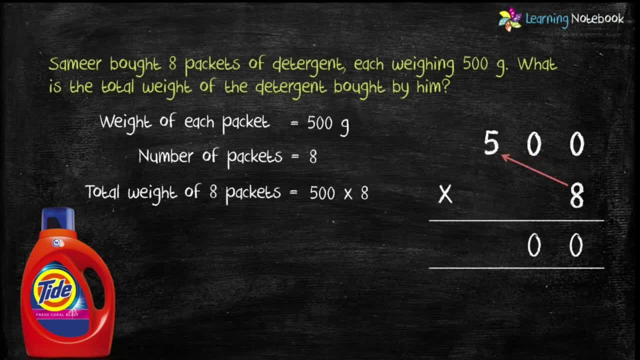 to 0 and 8 into 5 equals to 40. So we get the product as 4000 gram. Now, students, please remember that if the answer comes 1000 gram or more than 1000 gram, then always convert it into kilogram. So let's convert this 4000 gram into kilogram by dividing by 1000. So 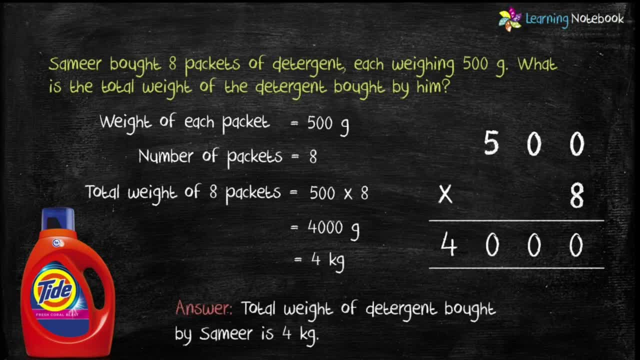 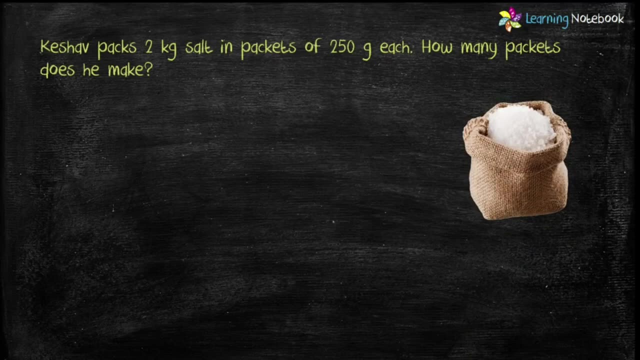 we get the answer as 4 kilogram Answer statement would be: total weight of detergent bought by Sameer is 4 kilogram. Question 4 is: Keshav packs 2 kilogram salt in packets of 250 gram each. How many packets does he make Students? let's write the statements: Weight of each. 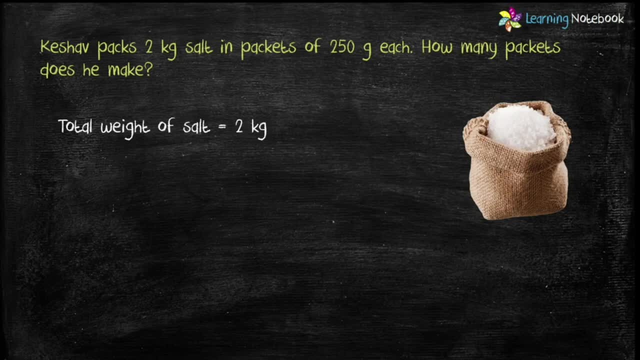 packet is 800 gram. Remember, total weight of salt is 2 kilogram and weight of each packet is 250 gram, Students, since we are given the weight of each packet in gram, so let's convert total weight given in grams. So to convert 2 kilogram into gram, we will. 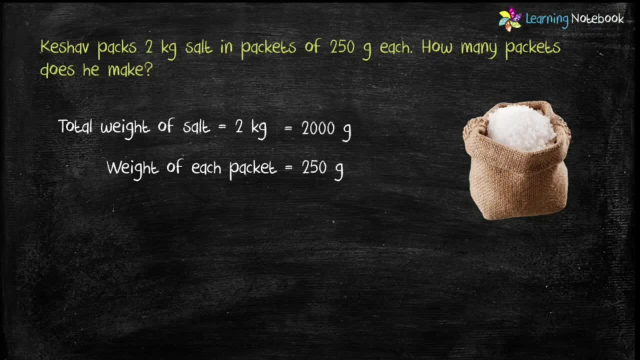 multiply by 1000. So we get 2 kilogram. Now let's write the statements. Weight of salt kilogram equals to 2000 grams. Now to find the number of packets made, let's divide 2000 by 250.. Cancel 0 by 0 and we get 200 by 25.. Simplify this and we get the answer as 8.. 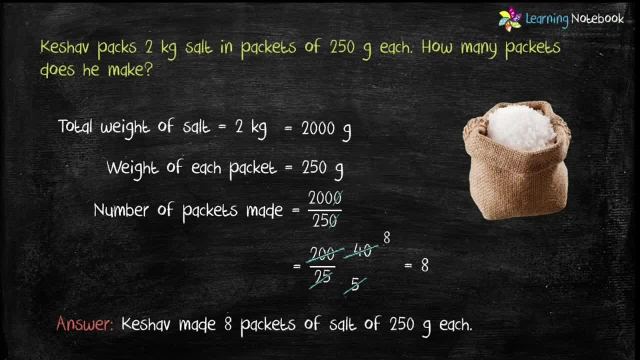 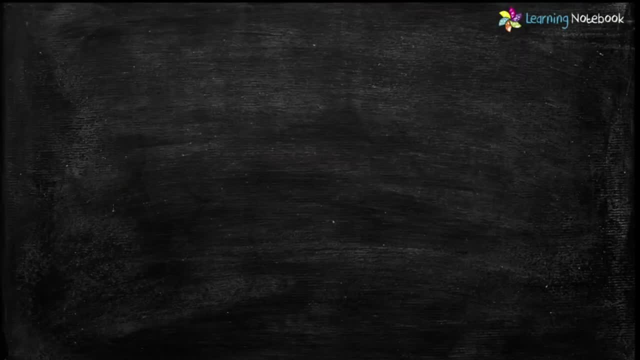 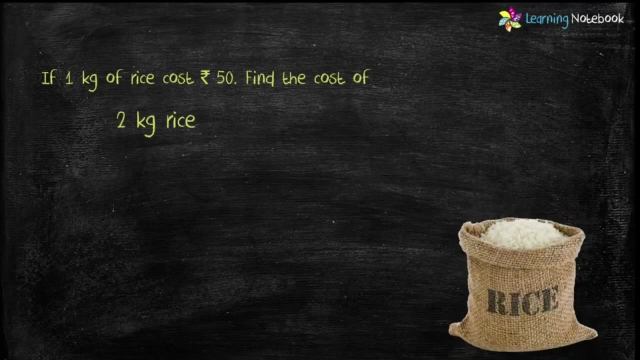 So answer statement is: Keshav made 8 packets of salt of 250 gram each. Next question is: if 1 kilogram of rice cost rupees 50, find the cost of first part is we have to find. 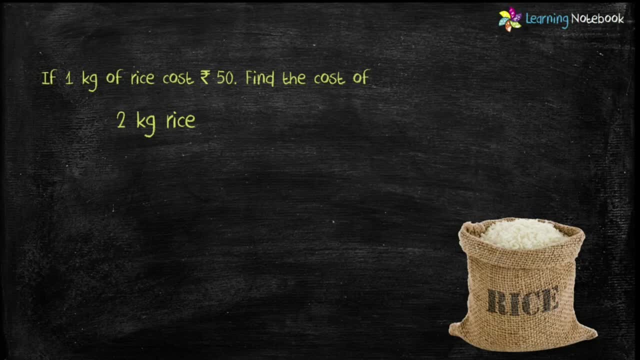 cost of 2 kilogram rice. Students. we are given cost of 1 kilogram rice equals to 1. And we have to find cost of 2 kilogram rice. It will be 2 into cost of 1 kilogram rice. 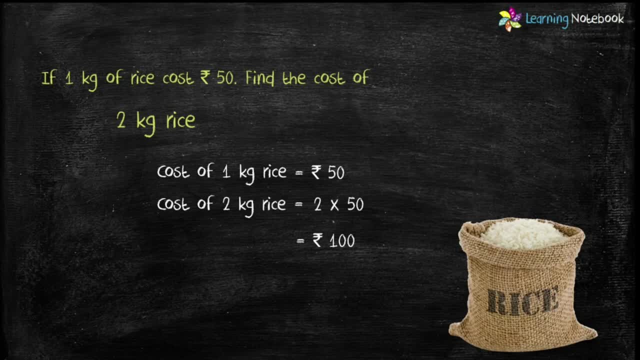 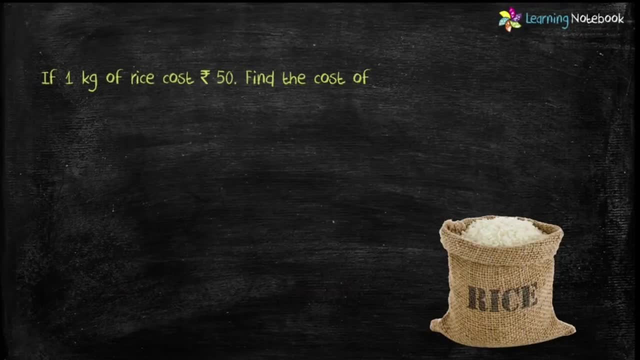 which is 50. So cost of 2 kilogram rice is 2 into 50, which is equals to rupees 100.. Now next part. we have to find cost of half kilogram rice. Again, students, cost of 1 kilogram rice equals to rupees 50.. So cost of half kilogram rice. 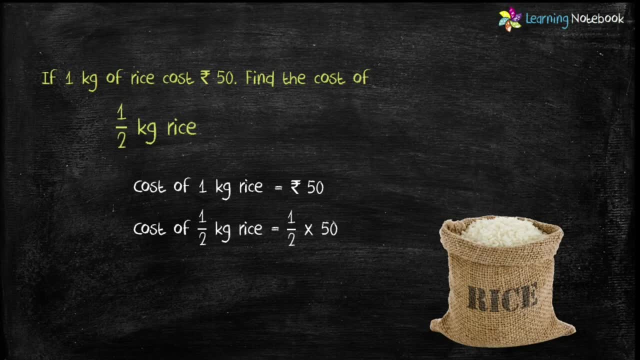 would be equal to half into cost of 1 kilogram rice. So it will be half into 50, which is equals to rupees 25.. So, students, cost of half kilogram rice is rupees 25.. Third part is find the cost of 100 gram rice. Here we need to find the cost of 100 gram. 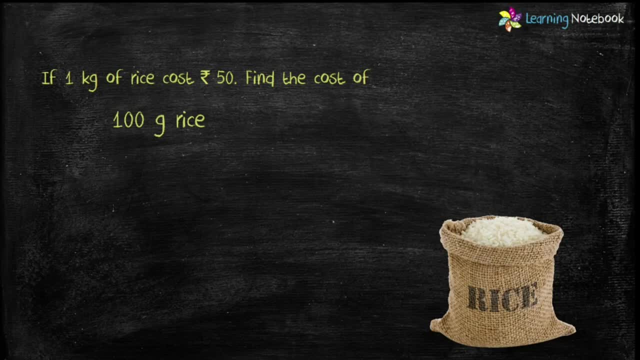 rice. Therefore it is not a direct question. In such questions we first find the cost of 1 gram and then we find the cost of 100 gram. So let's see how to solve this question. We are given cost of 1 kilogram. 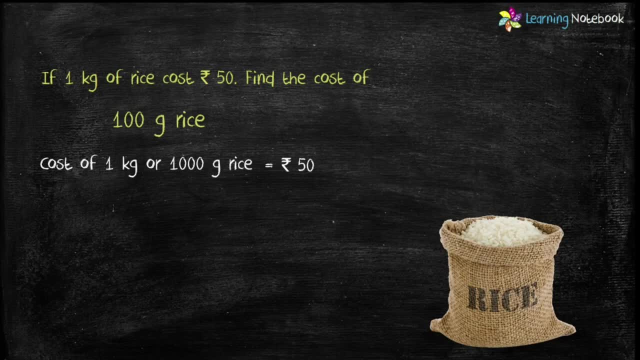 gram or 1000 gram rice equals to rupees 50. So cost of 1 gram rice will be 50 divided by 1000. Therefore cost of 100 gram rice would be cost of 1 gram rice multiplied by 100. So we get 50 divided by 1000 into 100.. Let's cancel 0 by 0 and we get the answer. 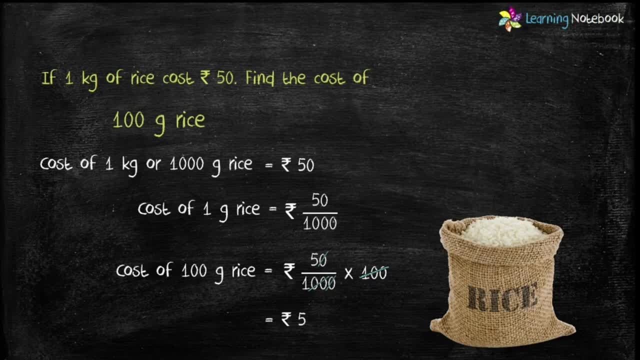 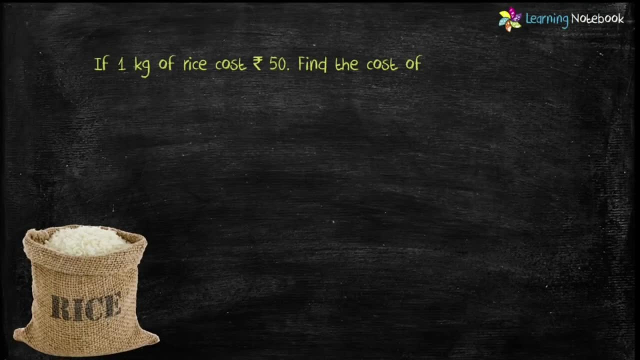 as rupees 5.. So students cost of 100 gram rice is rupees 5.. And the last part is: find the cost of 600 gram rice. Students. this is also not the direct question. Here also we will first find the cost of 1 gram. 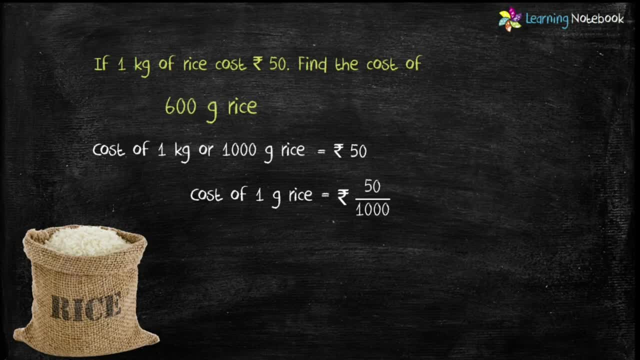 rice, which is equals to 50 upon 1000.. Therefore, cost of 600 gram rice will be cost of 1 gram rice multiplied by 600.. So we get 50 upon 1000 into 600.. Cancel 0 by 0 and we get the. 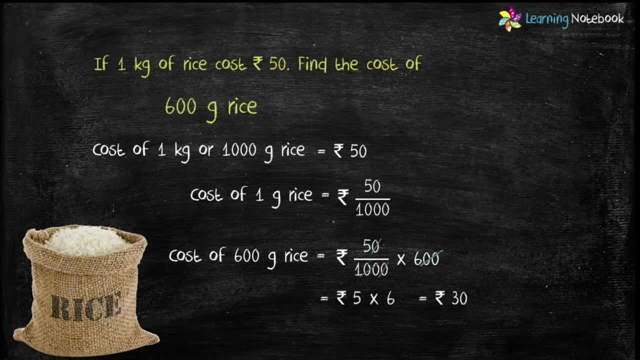 answer as rupees 5.. So, students, cost of 1 gram rice will be cost of 1 gram rice multiplied by 0. And we get 5 into 6, which is equals to rupees 30.. So, students, cost of 600 gram. 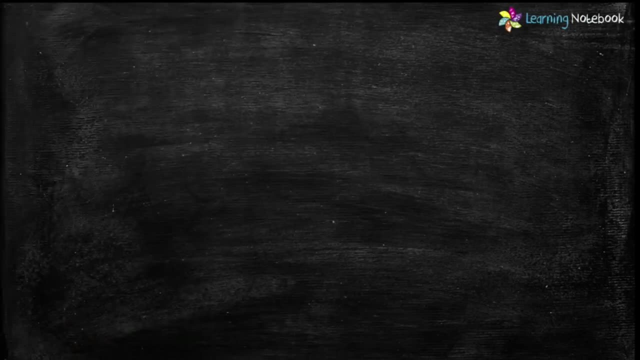 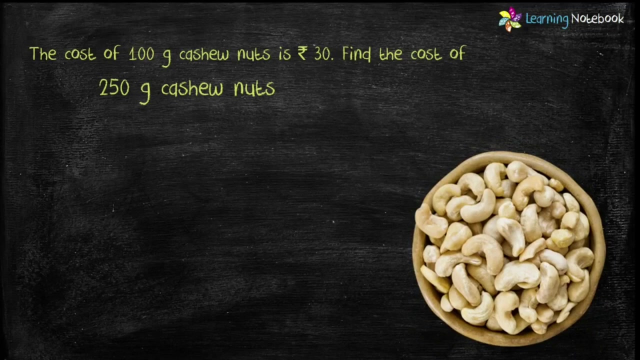 rice is rupees 30. Next question is: the cost of 100 gram cashew nuts is rupees 30. Find the cost of First part. is 250 gram cashew nuts? Students, now you know the cost of 1. you know how to solve such questions. first we will find the cost of 1 gram. 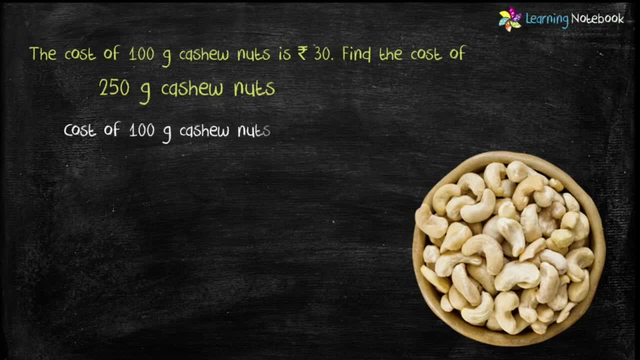 cashew nuts. so let's solve it. cost of 100 gram cashew nuts equals to the piece 30, so cost of 1 gram cashew nuts would be 30 upon 100. therefore, cost of 250 gram cashew nuts will be cost of 1 gram cashew nuts multiplied by 250, which is 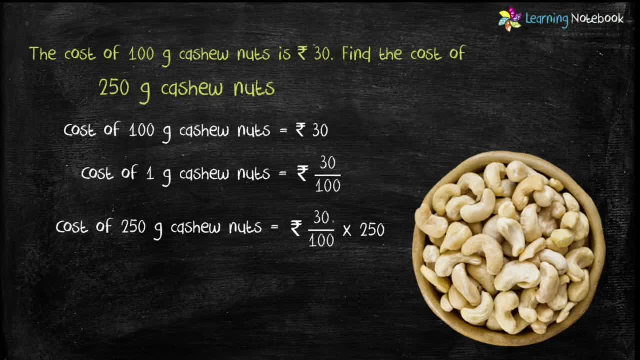 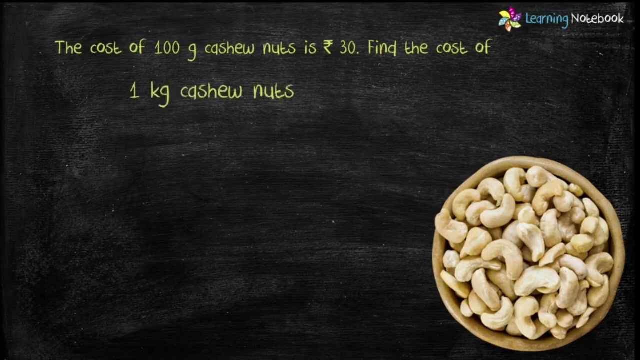 equals to 30 upon 100 into 250. cancel 0 by 0 and we get 3 into 25, which is equals to rupees 75. so cost of 250 gram cashew nuts is rupees 75. last part is: find the cost of 1 kilogram cashew nuts. so, students, let's solve it.